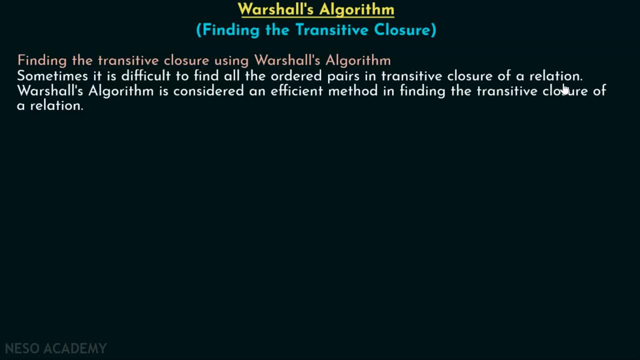 pairs in a transitive closure of a relation by brute force method. We can also find the transitive closure of a relation using Warshall's algorithm, and let me tell you, Warshall's algorithm is considered an efficient method in finding the transitive closure of a relation. Okay, that is. 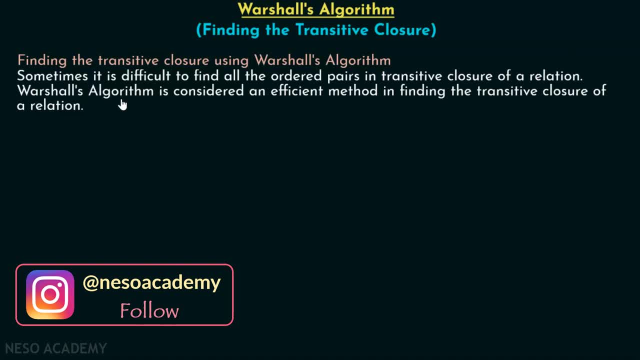 why we will use this algorithm, that is, Warshall's algorithm. Okay, here in this presentation, we will learn how to find the transitive closure of the relation using Warshall's algorithm, and we will learn this with the help of an example: By using Warshall's algorithm, find the transitive closure. 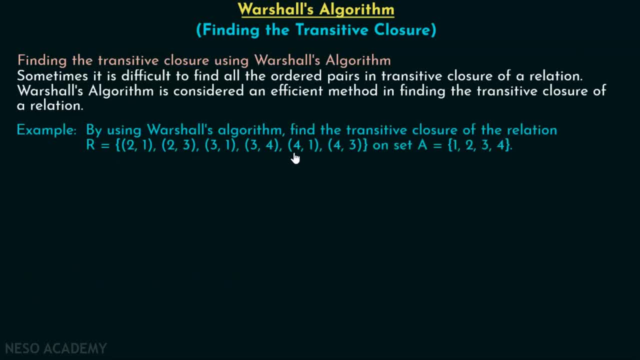 of the relation R, which consists of these ordered pairs, and this relation is defined on set A, which consists of these elements: 1,, 2,, 3, 4.. So we have relation R, which consists of these ordered pairs, and we have set A, which consists of these elements: 1,, 2,, 3, 4.. In order to apply Warshall's, 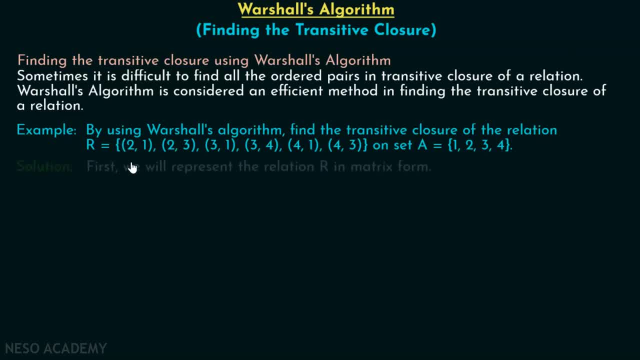 algorithm on this relation. first, we have to represent this relation in matrix form. Okay, we will represent relation R in matrix form Here. you can see this is relation R. Okay, currently we have no elements in this particular matrix. You can see that I have written 1,, 2,, 3,, 4 here, and 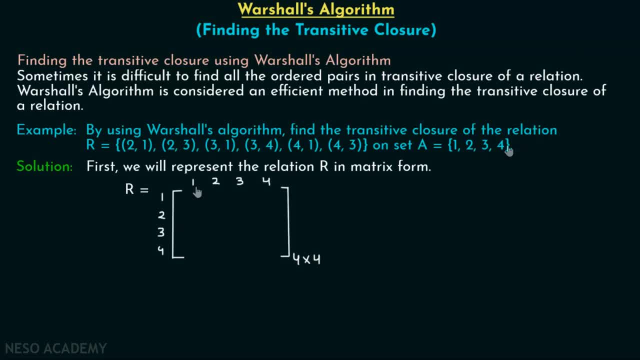 1,, 2,, 3, 4 here. These are all the elements of set A. We have to write them down on the top, as well as 1,, 2,, 3, 4.. First you can see we have to represent this ordered pair 2, 1.. This ordered pair is within: 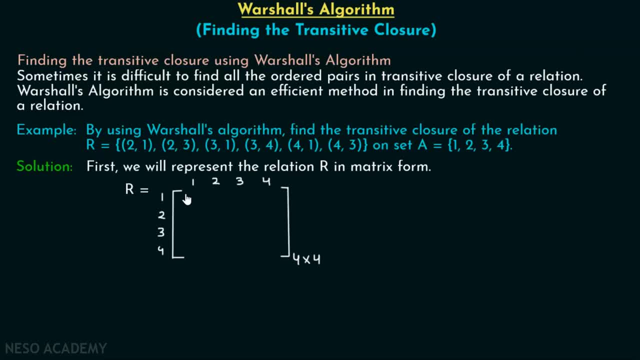 this relation R, In order to represent this ordered pair in this matrix, we have to place 1 over here. in this particular position, This is 2, 1.. Start reading from here and then you can read this particular element: This is 2, 1 and in this particular position, you have to place 1. 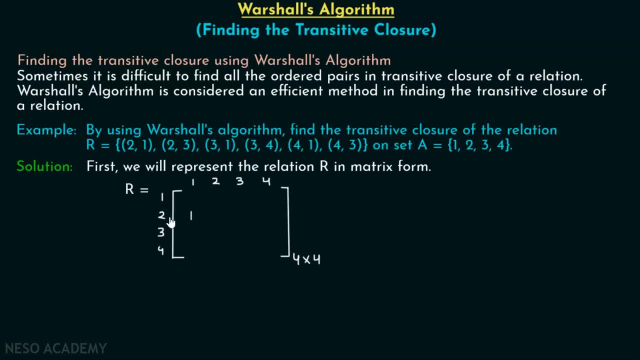 because we have to represent this ordered pair: 2, 1.. After this, we have to represent 2, 3.. So 2, 3 is this particular position? So let me place 1 over here. Then we have 3, 1.. 3, 1 is this? What about 3, 4?? 3, 4 is this position? 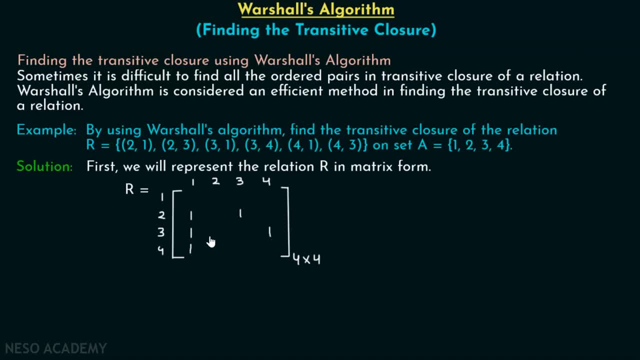 We will place 1 over here, Then we have 4, 1 and then we have 4, 3.. And in the rest of the positions we will place 0.. Okay, which means that 1, 1, 1, 2, 1, 3 and so on are not part of this relation. Okay. 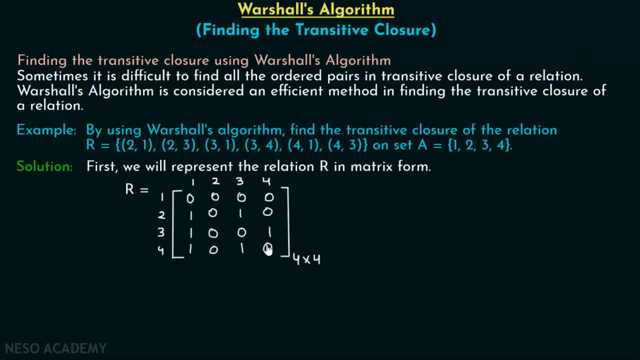 that is why I'm placing 0.. Okay, so we have 3, 1, 1, 2, 1, 3 and so on are not part of this relation. Okay, that is why I'm placing 0.. 0 over here. Fine, This is our matrix and this is. 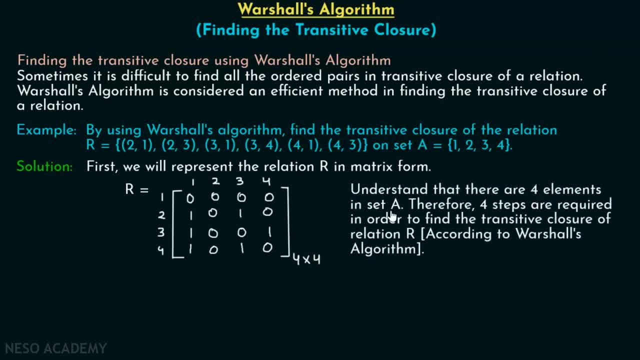 relation R. Understand that there are 4 elements in set A. Please see this: that there are 4 elements in set A. Therefore, 4 steps are required in order to find the transitive closure of relation. This is according to Warshell's algorithm. 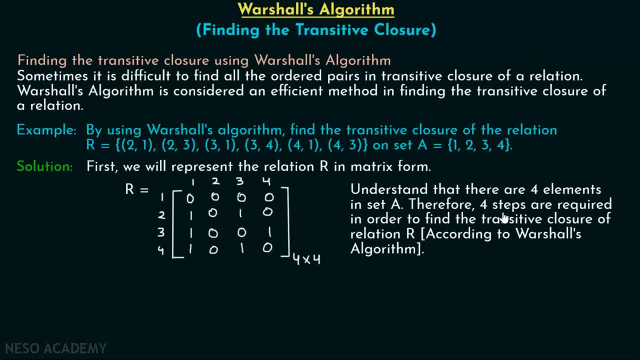 Now what Warshell's algorithm says. it says that number of steps actually depends on the number of elements in a particular set. Here we are considering the set A Right and relation R is defined on this set. There are four elements in this set. therefore, four steps are required in order to find the. 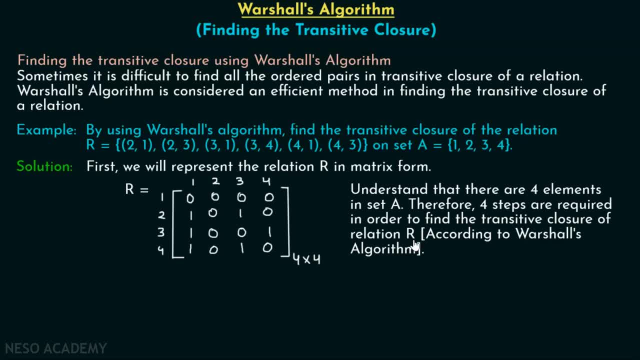 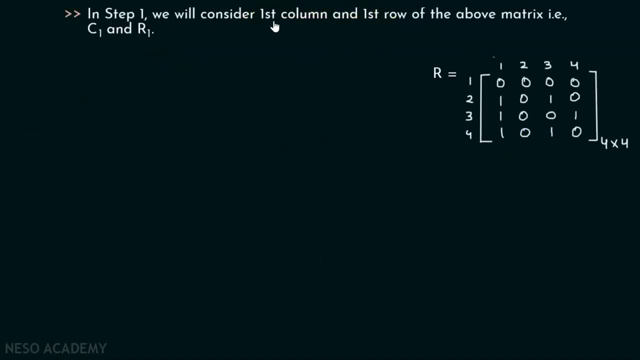 transitive closure of relation R. This is according to Warshall's algorithm. Now we will discuss all four steps one by one. Here is step number one. In step one we will consider first column and first row of the above matrix. I have redrawn the matrix here. okay, We have to consider first. 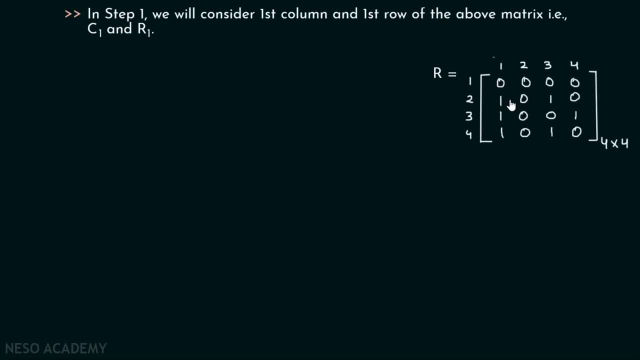 column and first row of this particular matrix. This is according to step one. okay, Let me represent first column by C1 and first row by R1, okay, So C1 represents first column and R1 represents first row. We have to consider first column and first row of this particular matrix. 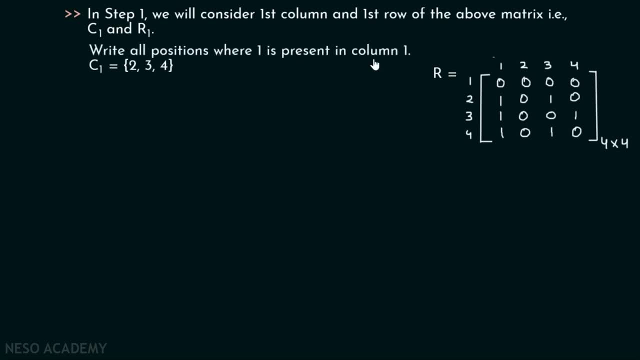 okay, Now we have to write all positions where one is present in column one. okay, You can see that one is present in position two, position three and position four. So it is clear that C1 is nothing but two, three, four, right? So C1 is. 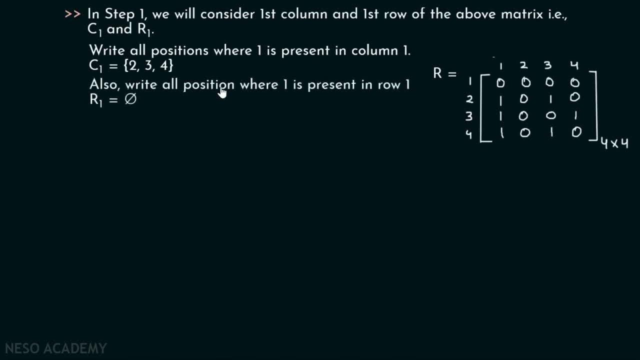 equal to two, three, four. After this we have to write all positions where one is present in row one. You can see that one is not present anywhere in this particular row, right? Therefore R1 is phi. okay, Now we have to take the cross product of C1 and R1.. So C1 cross, R1 is obviously phi. 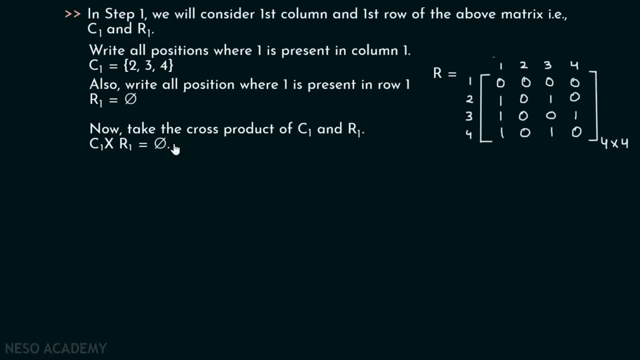 because R1 is phi. Phi cross with anything is always phi. Therefore there are no new additions. I'll tell you what is the meaning of additions, But right now you should understand that C1 cross, R1 is phi. Therefore there are no new additions. okay. 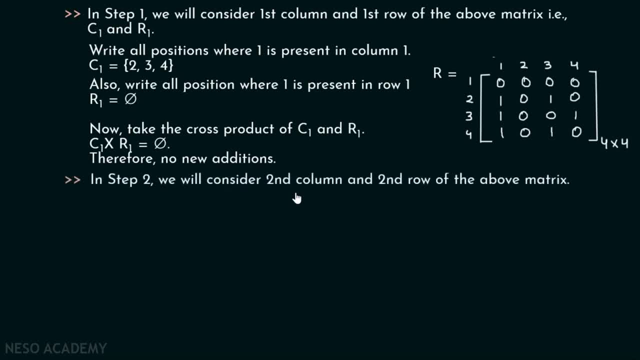 Now we will consider step two. In step two we will consider second column and second row of the above matrix, that is, this matrix. Let's consider second column and second row of this matrix. You can see that in second column we have no ones present. Therefore, C2 is phi, and 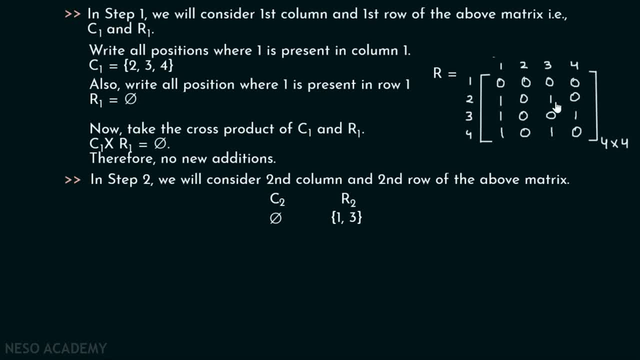 in R2, we have one present over here as well as here, And you can see that this is position one and this is position three. Therefore, R2 is nothing but one comma three. What is C2 cross R2? C2 cross R2 is nothing but phi, because C2 is phi. Therefore, no new additions, okay. 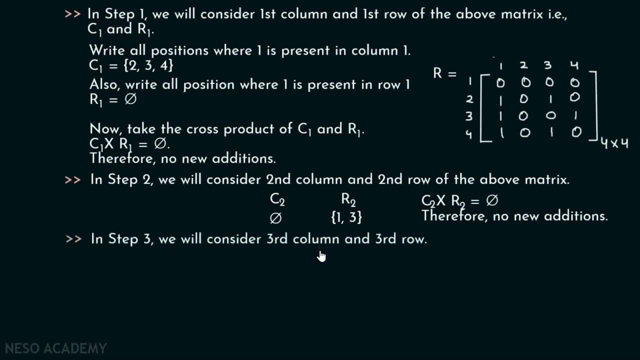 Now we will discuss step three. In step three, we will consider third column and third row. okay, Let's consider third column and third row. In third column, you can see that one is present in position two and position four, And in third row, we can clearly see that one is present in position one and position four. 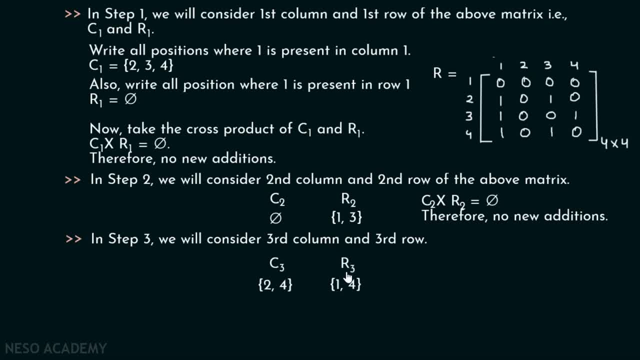 So let me just write them down over here: C3 is nothing but two, four and R3 is nothing but one, four. What is C3 cross R3?? C3 cross R3 is nothing but two, one, two, four, four, one, four, four. 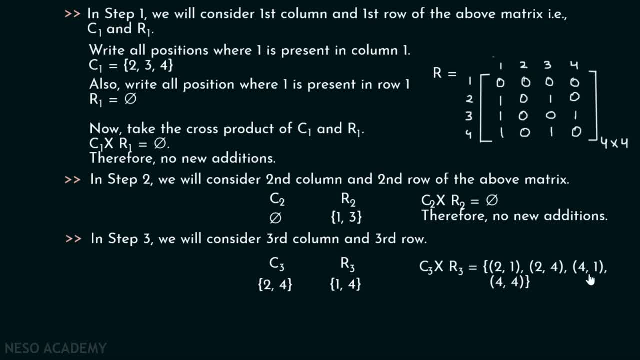 That's what I have written over here, Obviously, on ordered pairs form. Now you can see that C3 cross R3 is not five. Actually, what we have to do now, according to Warshall's algorithm, we have to place one in these positions. 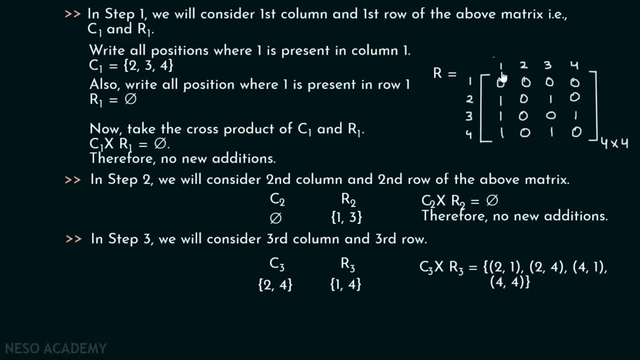 This means in position two, one that is in this particular position, you have to place one Already. one is present over here. In position two: four, you have to place one. In position four: one you have to place one. One is already present. 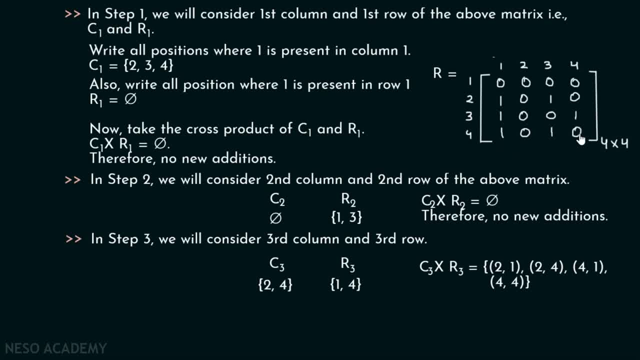 In position four, four in four four also, you have to place one. That is why I have told you, in these two cases there are no new additions. But in this case we have to put one in all these positions And you can see we have two new additions. 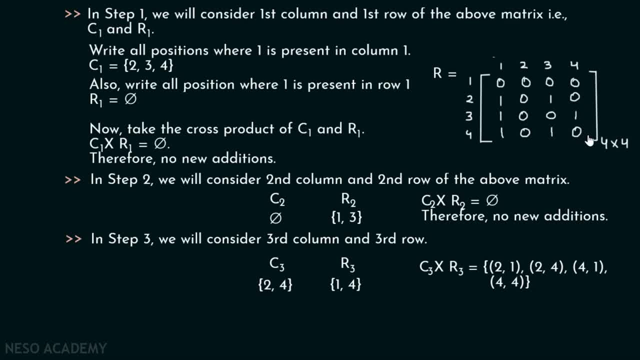 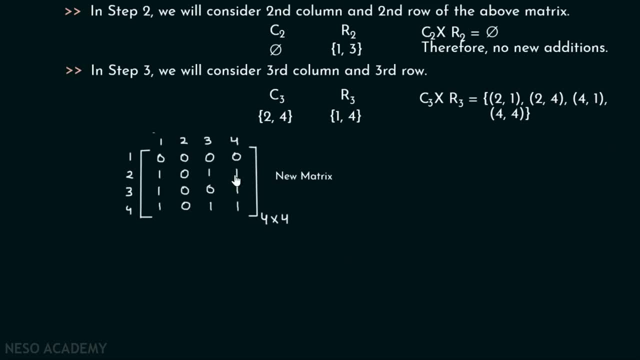 We have to replace this zero by one and this zero by one, And this is how new matrix looks like. Okay, you can see that I have placed one over here and one over here. Rest of the matrix is similar to what we have seen already, right? 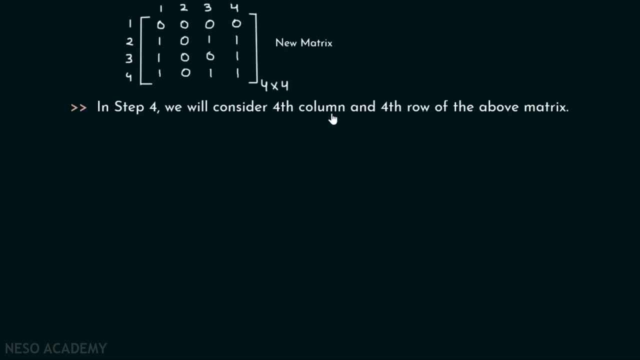 Now we will discuss step four. In step four we will consider fourth column and fourth row of the above matrix. Here we have to consider fourth column and fourth row of this matrix. You can see that C4 is nothing but two, three, four. 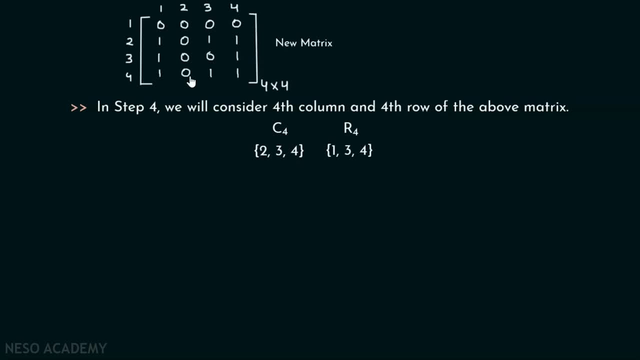 That's what I have written over here. And R4 is nothing but one, three, four. That is what I have written over here. And what is C4 cross R4? Two, one, two, three, two, four, three, one, three, three, three, four, four. one, four, three, four, four. 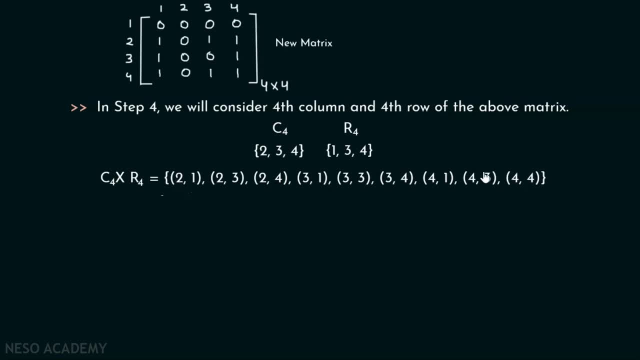 Right, We have to place ones in all these positions. Let's place one over here in two, one, then two, three, then two, four, Then three, one, three, three, three, four, four. one, four, three, four, four right. 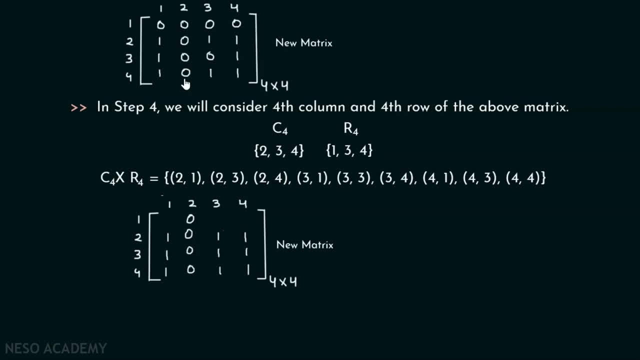 Here we have to place all zeros, as you can see over here. We have to place zero over here as well. right? This is how new matrix looks like. right, And let me tell you: this is nothing but R T plus. This is nothing but R T plus. 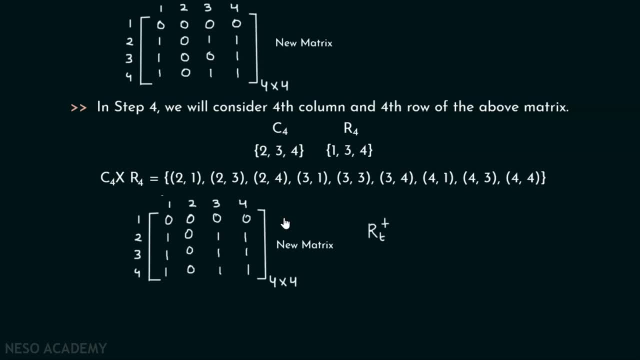 Right, This is the transitive closure of relation R. I have told you that we have to find the transitive closure using Warshall's algorithm and, according to Warshall's algorithm, if there are four elements in a particular set, then four steps. 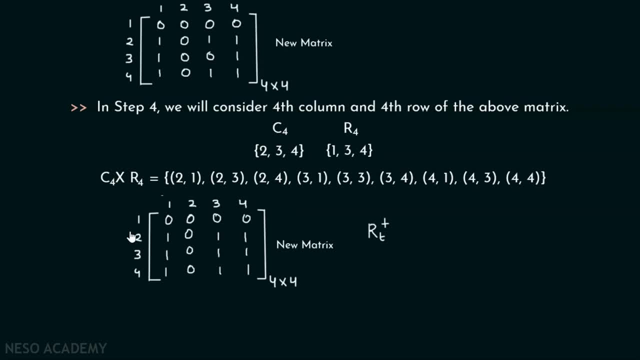 are required. We have completed all the four steps and this is what we have obtained. This is R T plus, right. R T plus is nothing but two, one, two, three, two, four, three, one, three, three, three, four, four. one, four, three, four, four. 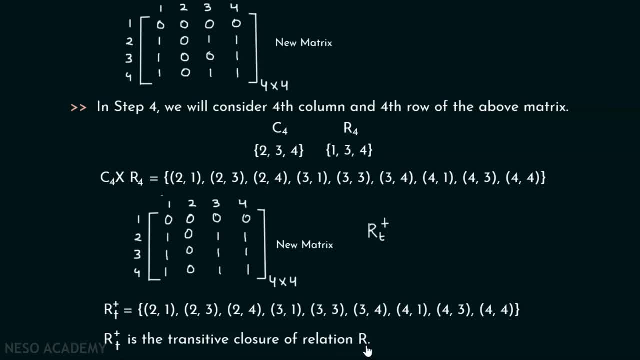 As simple as that. And let me tell you. this is the transitive closure of relation R. Okay, This is all about Warshall's algorithm. According to Warshall's algorithm, first you have to represent your relation R in matrix form, and then you have to see how many elements are there in particular set on which that. 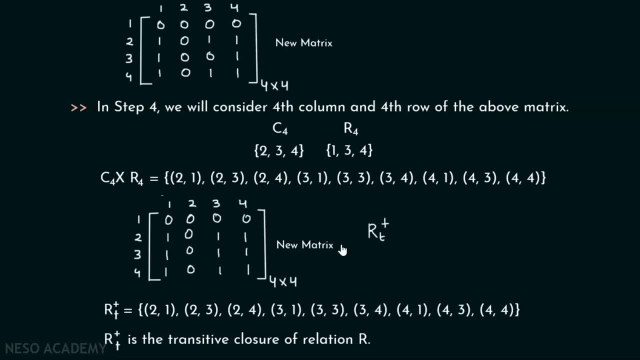 relation is defined. Okay, As you can see, in this particular example we have set A and in set A we have four elements: one, two, three, four. As there are four elements in set A, therefore, four steps are required in order to find the.